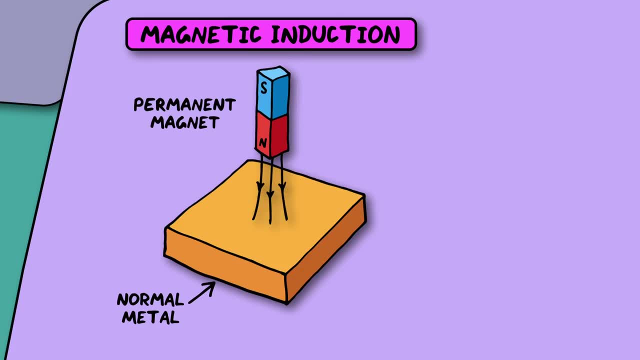 They feel a force from it and start moving in a circle called an eddy current. This is called magnetic induction. In a normal metal, this current dies away quickly because the material has got electrical resistance. The moving electrons bang into the atoms and stop moving. 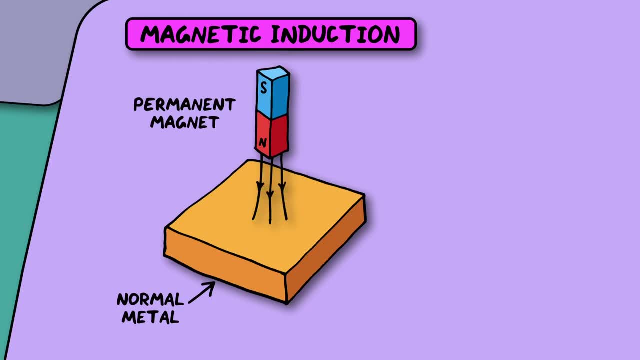 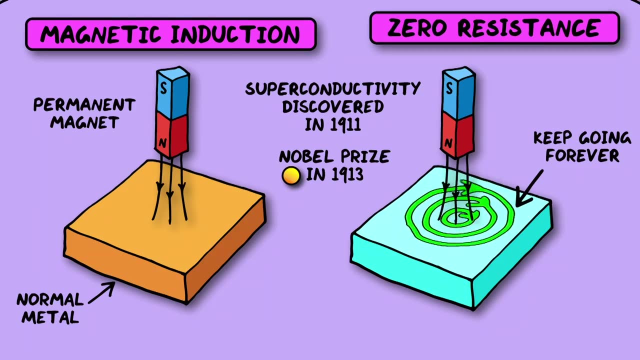 giving up their energy to vibrations in the atomic life. And if you do the same thing to a superconductor, because they've got zero electrical resistance, the eddy current will never stop flowing and will carry on circulating forever, Like age of the universe. forever according to the theory, And experimentally we've seen. 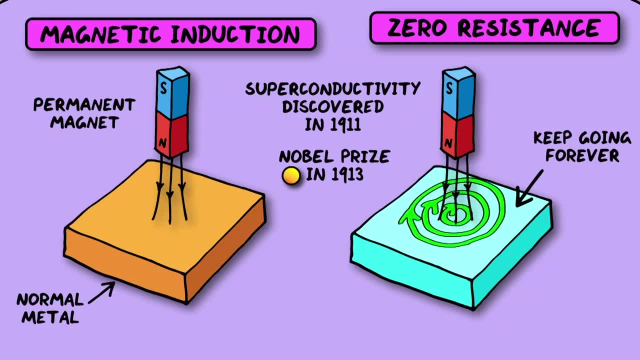 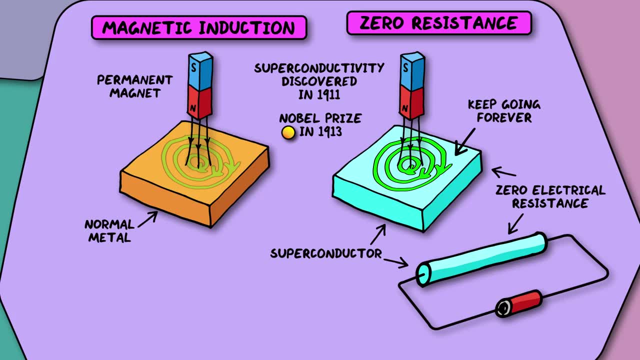 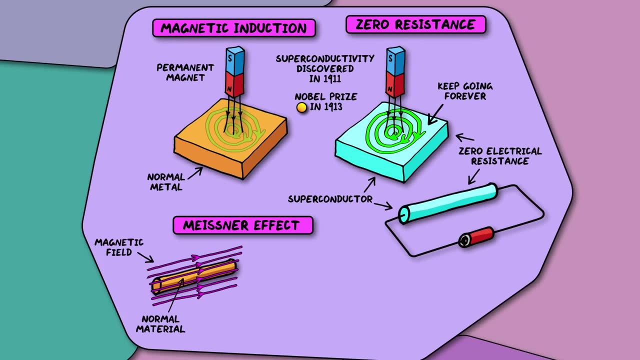 currents losing no energy over 25 years. Zero electrical resistance also means you can pass a direct current through a superconductor without it losing any energy at all. That's cool, but the other important property to do with magnetic fields is called the Meissner effect. 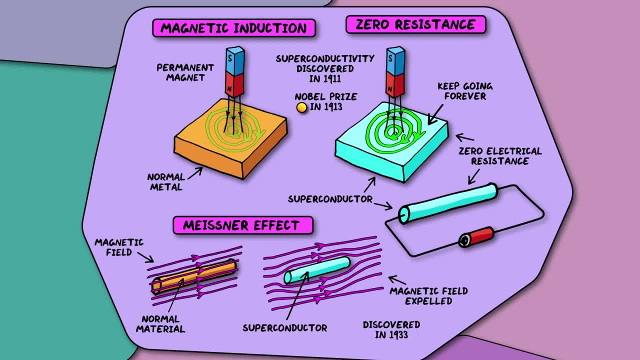 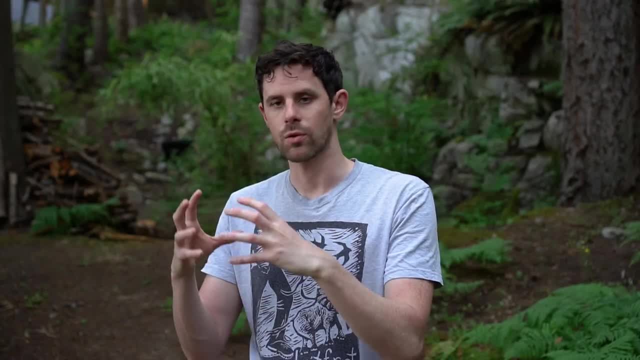 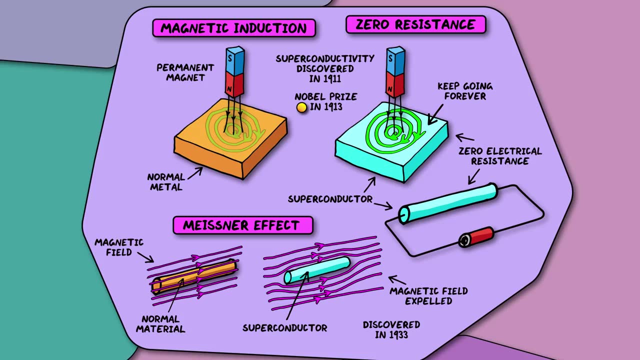 Superconductors expel any magnetic field inside them. You know how I said that magnetic fields induce electrical currents in conductors. Well, the opposite is also true: Any electrical current creates a magnetic field. If a superconductor is in a magnetic field, it gets a load of eddy currents which create 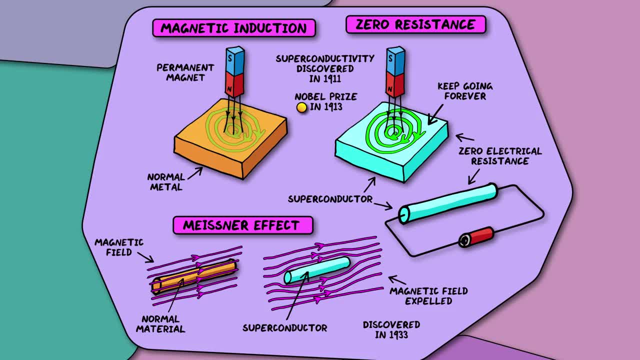 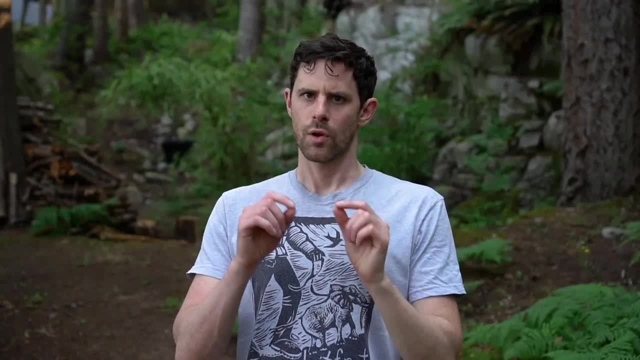 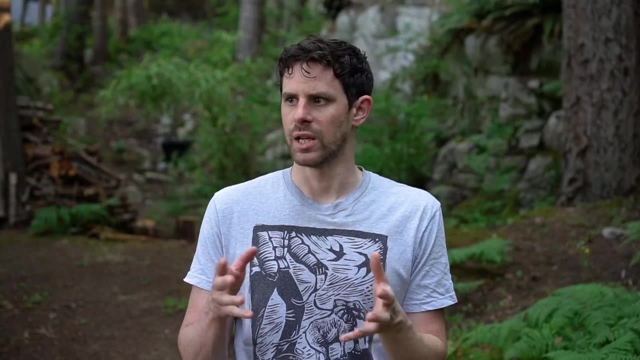 their own magnetic fields that exactly cancel out and expel the original magnetic field. This is a quantum effect and doesn't happen in normal conductors. So those are the two main features of superconductors- Zero electrical resistance and the Meissner effect- And when they were discovered in the early 1900s, physicists were: 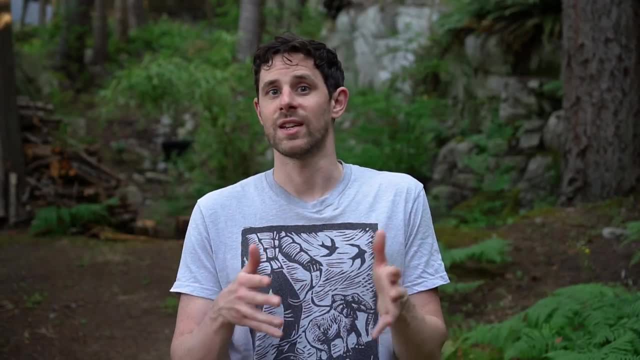 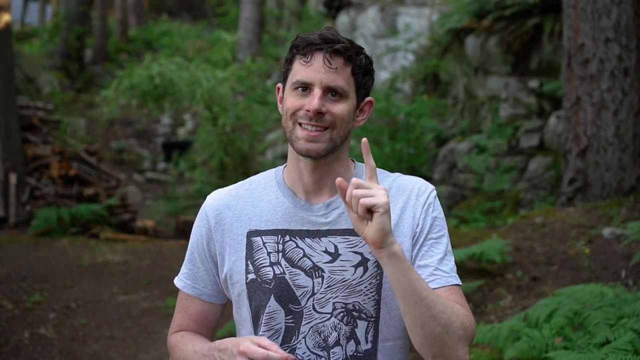 like whoa, And then since then they've investigated more and made a load of useful technology out of them, which we'll look at in a bit. But first we need to look at exactly what conditions are needed for a superconductor to superconduct. 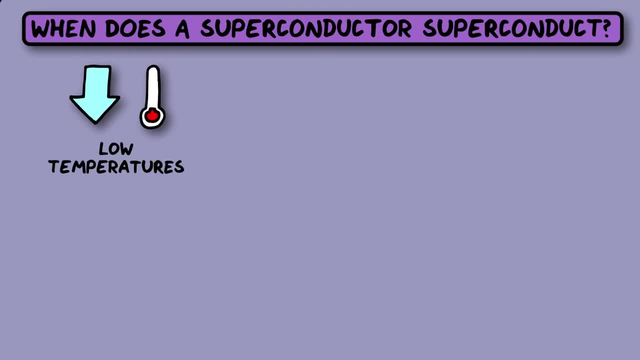 There are three conditions you need for a superconductor: Low temperatures, small enough magnetic fields and small enough electrical currents. Although these two are kind of the same thing, The specific temperature and magnetic field that breaks superconductivity depends on the material. 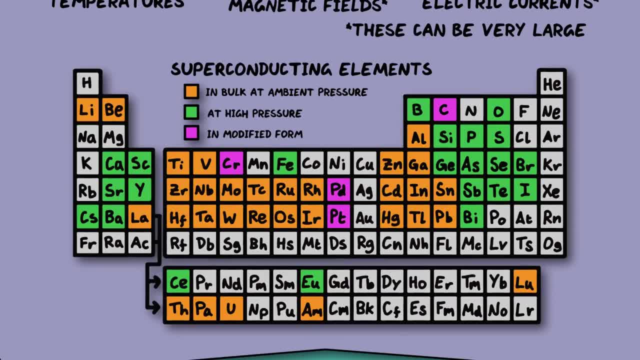 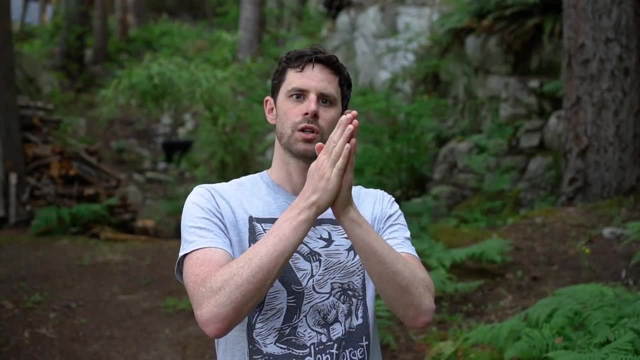 The first superconductors that were studied were pure elements like mercury, aluminium or niobium, and physicists discovered that not all of the elements superconduct. Here are the ones that do For each material, as you cool them down, they undergo a sharp transition temperature where 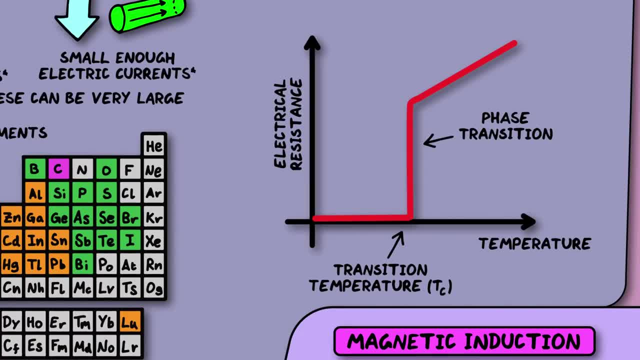 they suddenly start superconducting at a sharp phase transition. And when they're in the superconducting state, if you then apply a larger and larger magnetic field or a larger and larger electrical current, they've got a critical field and a critical current where they suddenly stop. 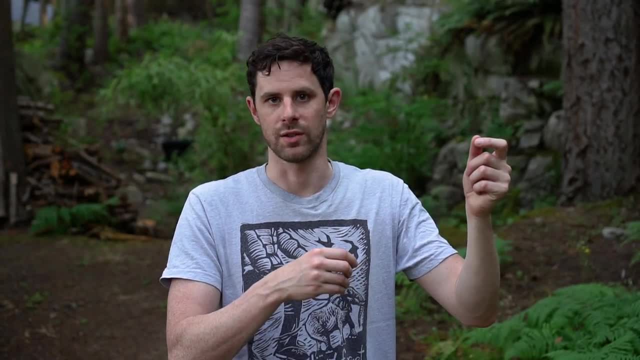 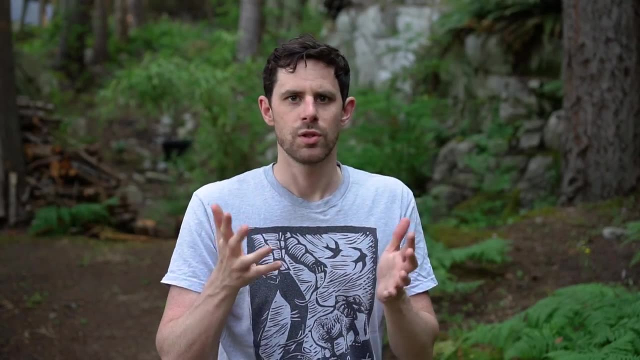 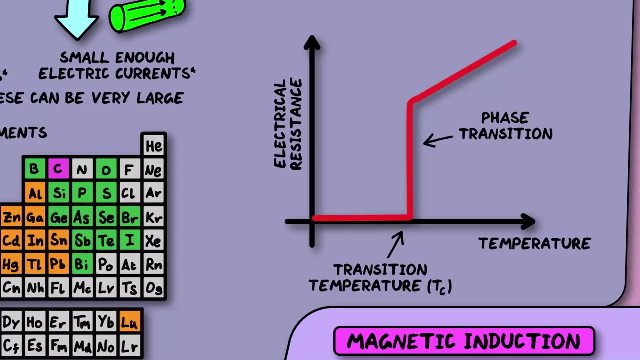 superconducting and go back through the phase transition to a normal conductor, even if they're below the transition temperature. Now, even if this is all new to you, you already know about phase transitions, because this is what happens to water when it freezes or when it boils. These are phase transitions too, but these are phase transitions in the material. 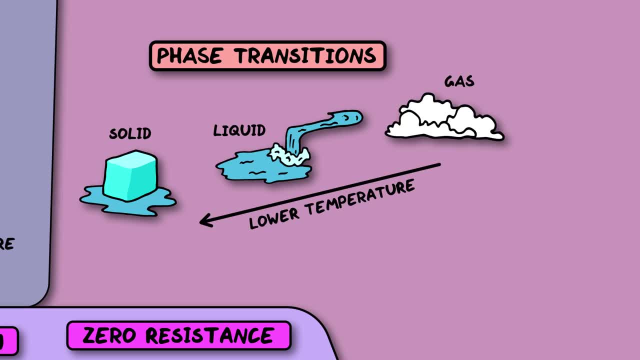 properties, whereas the superconducting phase transitions are transitions in the electronic properties. But it all comes down to what is the configuration of stuff which minimizes the overall energy, known as the Gibbs free energy, If a material will be in a lower energy by freezing into a solid or turning into a superconductor. 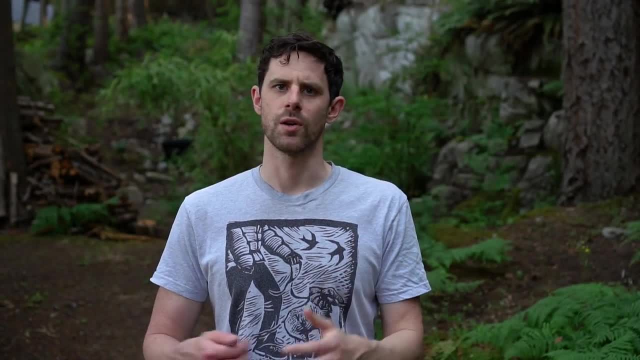 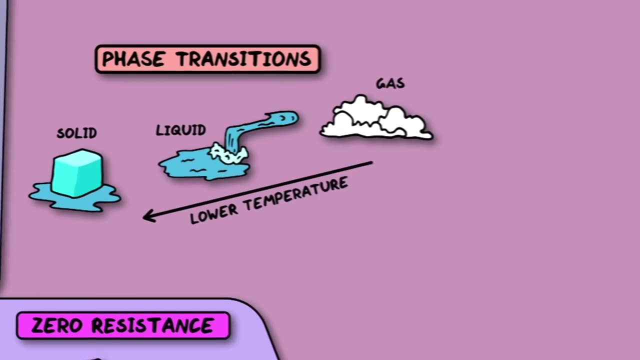 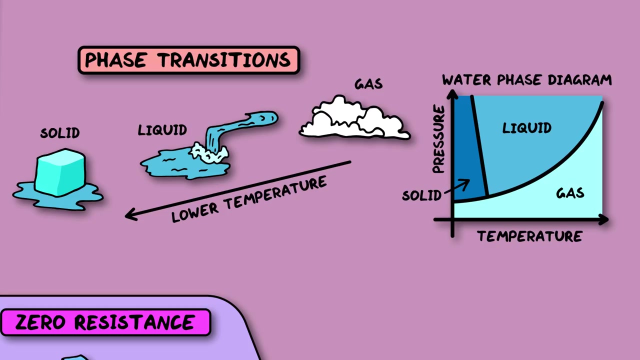 that's what it'll do. Anyway, as any fan of physics knows, when we have phase transitions, we're going to have- say it with me- phase diagrams. These are very handy graphs because they show us what state your thing will be in when you change some global parameters. This is a phase diagram for the state. 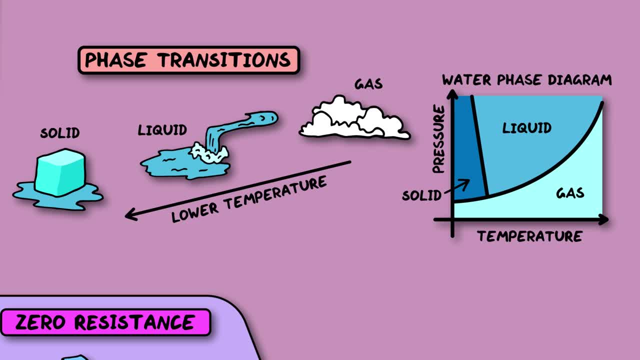 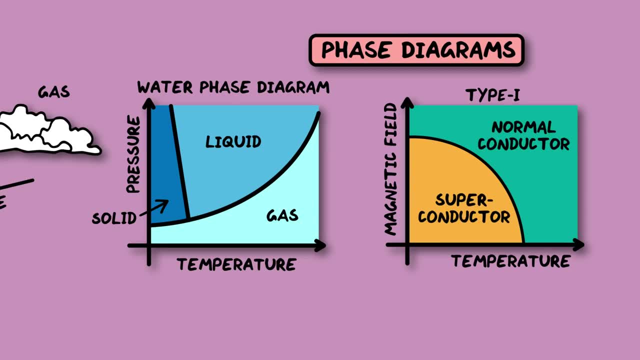 of water. when you change temperature and pressure, which you might have seen before, And here is the analogous example of the superconducting state and normal conducting state for different temperatures and magnetic fields of a superconductor, This also changes with pressure as well, but I'm not. 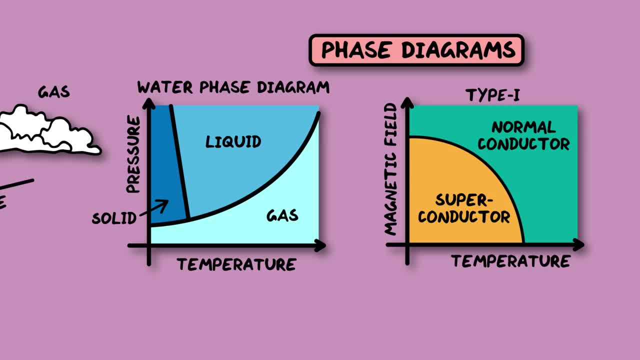 plotting that here because I'd need a 3D plot and superconductivity at pressure is a bit of a research niche. The vast majority of superconductors are used at normal pressure. Each superconductor has got its own unique phase diagram and filling them in kept a bunch of 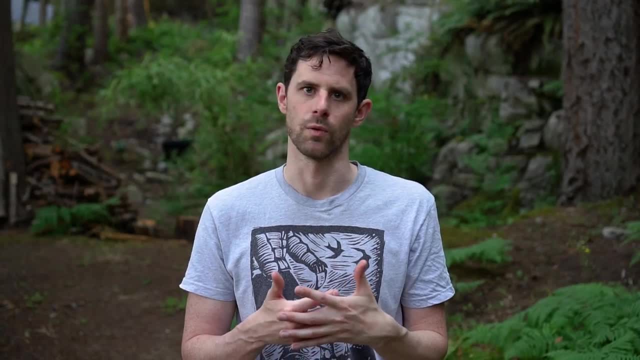 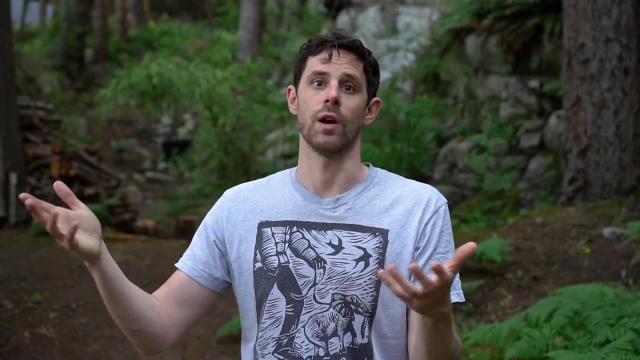 experimental physicists happily busy for years, as they filled in all the points And they didn't just stick to the elements. they started looking at compound materials, of which there are an infinite amount, and the search for new superconductors has been going on ever since in attempt to find 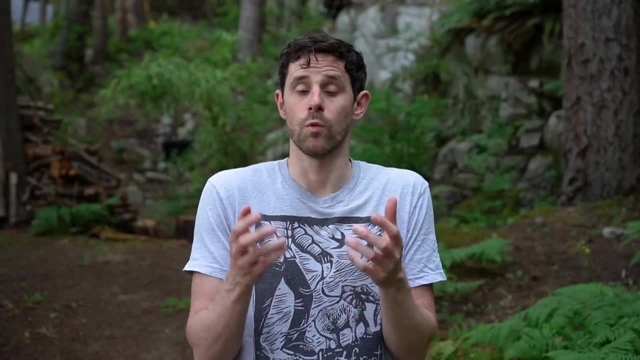 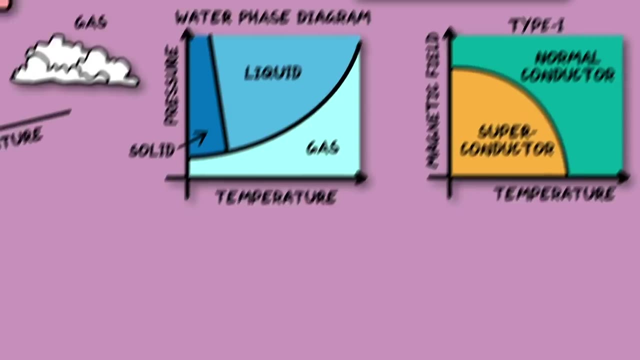 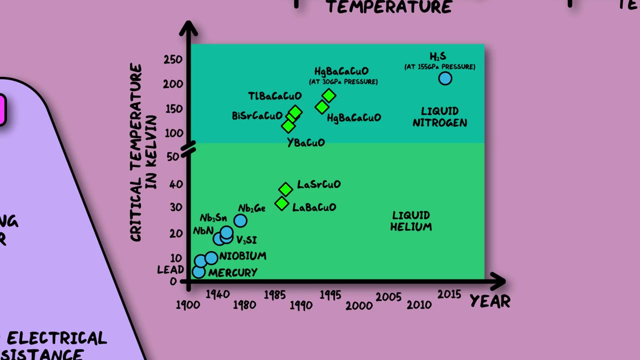 materials with higher and higher transition temperatures, with the goal of one day finding a room temperature superconductor and then making tons of cash. Here's a plot of the discovery of higher and higher temperature superconductors, and along the way they've made some startling discoveries. First of all, in 1935 they discovered 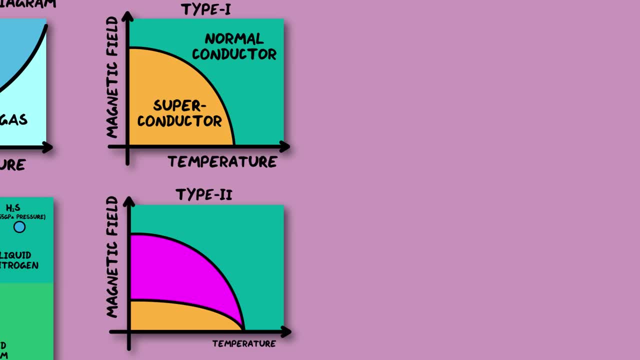 type 2 superconductors, which behave differently to the superconductors I've described so far, which were then called type 1 superconductors. Type 2 superconductors behave differently to type 1 superconductors when they're in a magnetic field. Here's a phase diagram of a type 2. 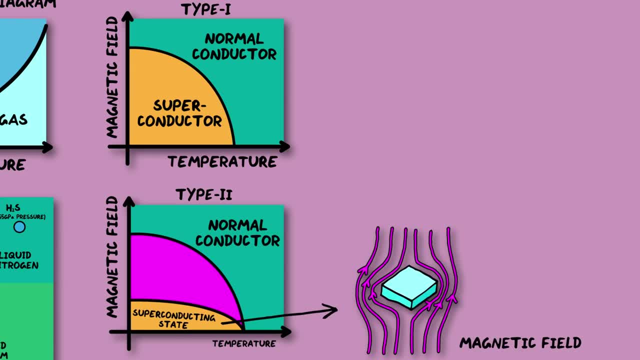 superconductor Down here it still behaves like a type 1 superconductor, but then they have an intermediate state where they do let the magnetic field flow. The magnetic field penetrates them, but only in specific points in a formation called a magnetic field vortex, or vortices for short. Here the bulk of the material is still superconducting. 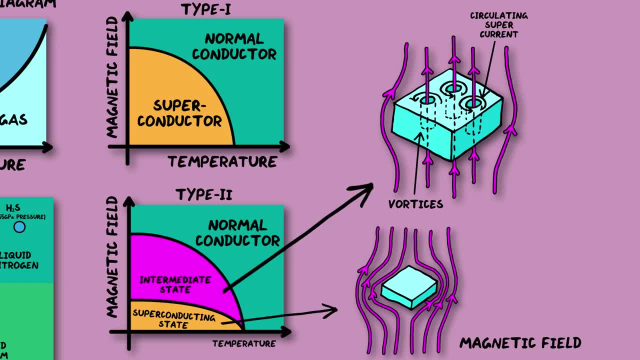 but at these thread-like vortices the material is a normal conductor. The magnetic field goes all the way through in a certain small amount, called a magnetic flux, quanta, and each one is surrounded by a swirling supercurrent, which is the name for the electrical current in a 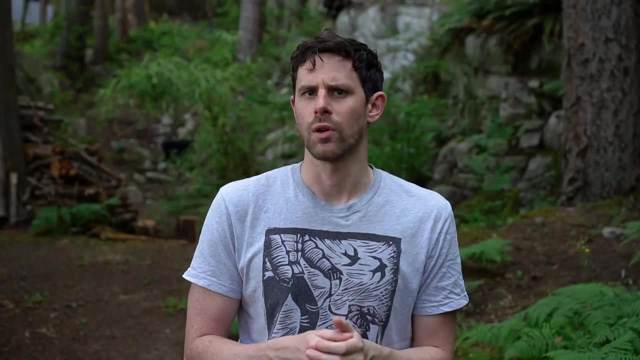 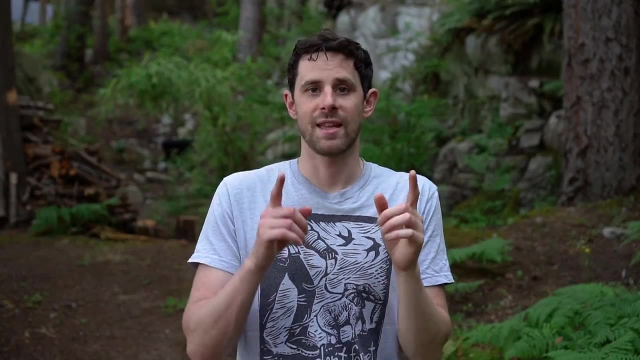 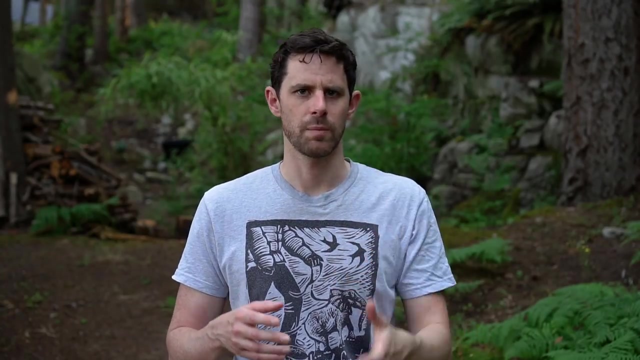 superconductor. I just threw a load of terminology at you there, so if you're confused, just think of them as a load of sausages And you'll be pleased to hear that these are the only two kinds of superconductors we've found so far. There is a kind of type 1.5 superconductor, but I can't be bothered to. 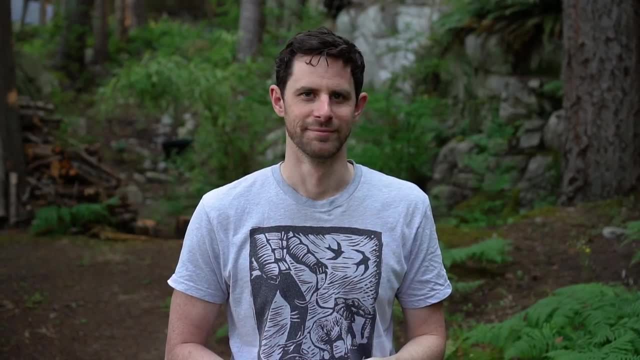 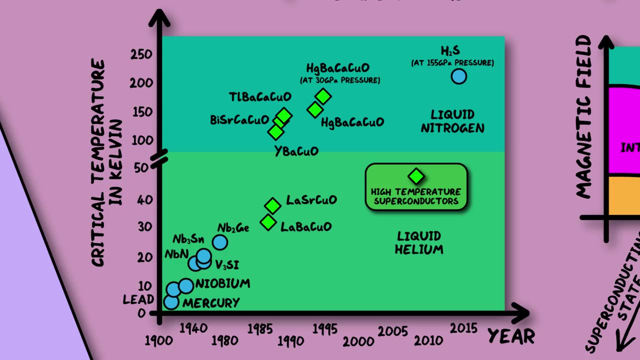 talk about it here. so Wikipedia. The next big bombshell to hit the exciting world of superconductivity research was in 1986, when researchers made a superconductor made of carbonic, which was an insulator before being cooled down. This then led to the discovery of 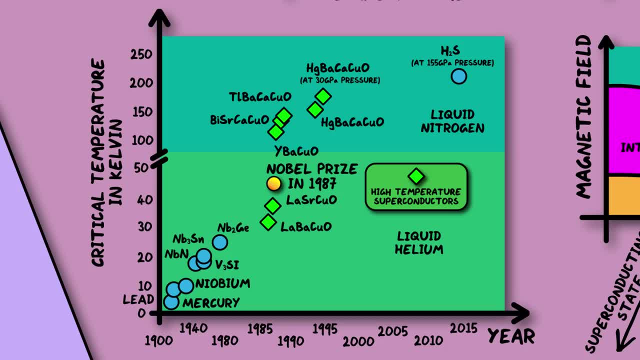 a bunch of high temperature superconductors, Although high temperature is a little bit of a misnomer because they still have to be cooled way below zero with cryogenic liquids. but now you can make a thing superconduct with just liquid nitrogen at 77 kelvin, which is way cheaper than 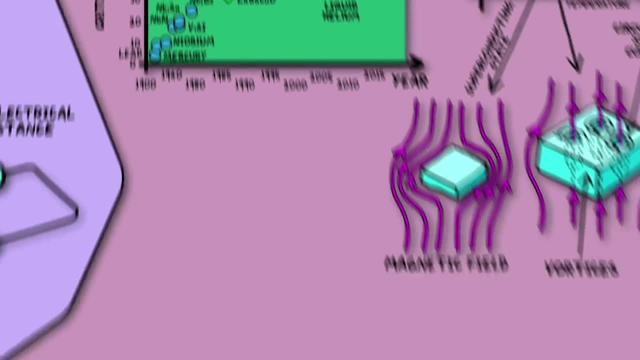 liquid helium, which is what they had to use before. These new superconductors are known as the cuprates because they contain layers of copper oxide. These new superconductors are known as the cuprates because they contain layers of copper oxide. These new superconductors are known as the cuprates because they contain layers of copper oxide. 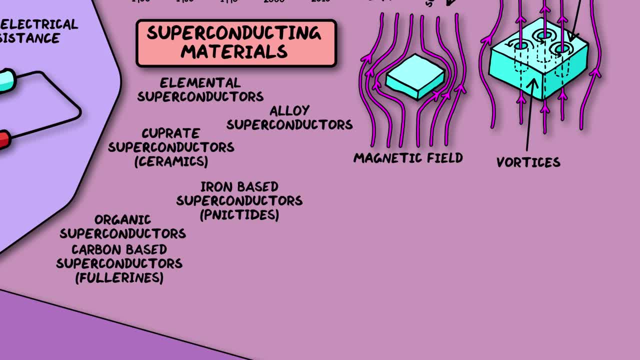 with a load of other stuff in there as well, and there's also many other types of superconductor: iron-based superconductors called the pinnictides, pure carbon-based superconductors called fullerenes and also known as organic superconductors, and there's others as well, but you get the picture. 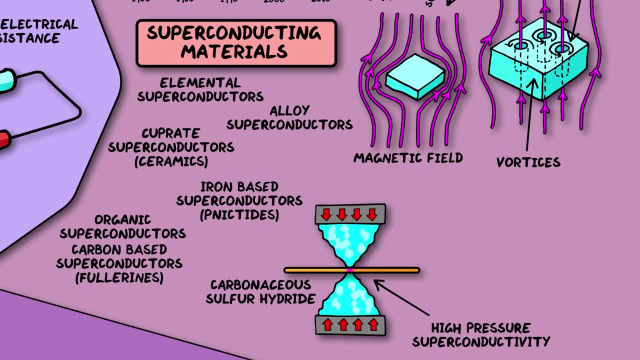 people have also squeezed materials between diamond presses and discovered that many materials start superconducting when they're at very high pressure, and recently, in 2020, a room temperature superconductor was discovered called gaseous sulfur hydride, which superconducts at 15 celsius, but only under a huge amount of pressure. 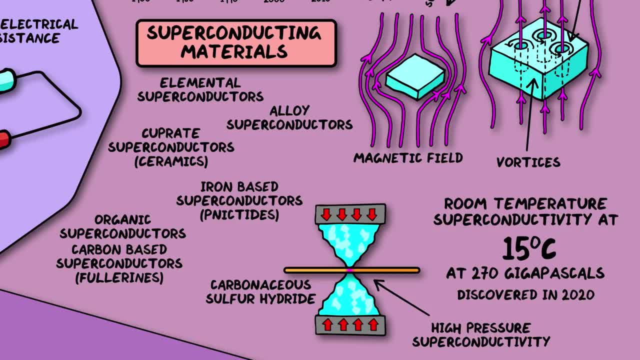 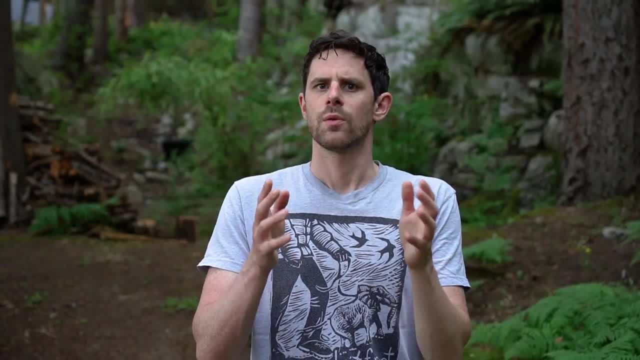 squeezed in a diamond press, so it's not actually practically useful, but still a landmark discovery. now onto the theory of superconductivity. it was not an easy job to figure out the underlying theory of what's actually going on in superconducting materials at the scale of 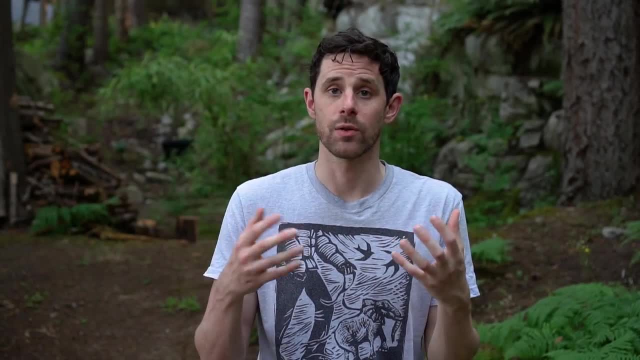 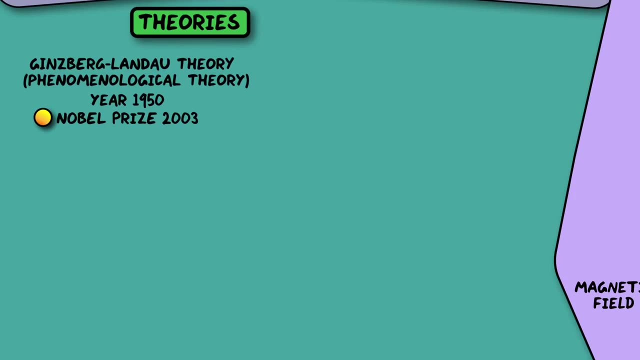 the electrons. what's the underlying process that allows for zero resistance? the first theory, ginsburg-landau theory, predicted properties of superconductors like which would be type 1 and type 2, but this was superseded by a microscopic theory called bcs theory, named after the initials. 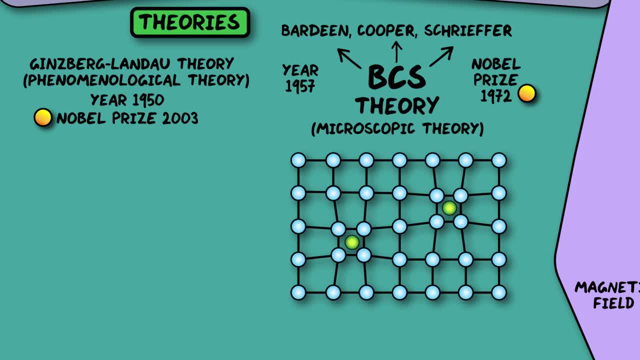 of the creators. they figured out that as electrons move through the lattice of atoms, they attract the atoms around them slightly, creating a local positive charge which creates an attractive force between electrons. so electrons can interact with each other through vibrations- the lattice called phonons, and this allows them to pair up in a composite entity known as a cooper. 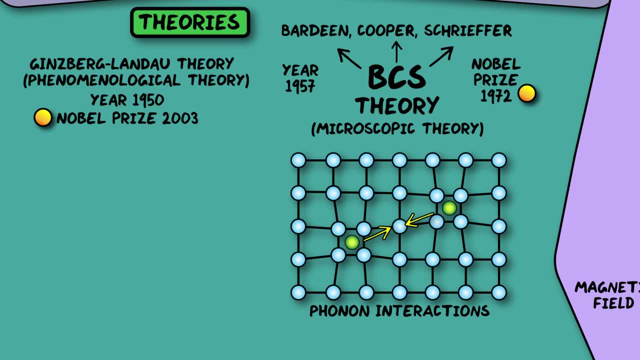 pair. now if you've watched my map of particle physics, you'll know that electrons are spin half particles and obey the powerly exclusion principle, so can't exist in the same quantum states. but the cooper pairs behave like bosons because when you add their spins together you get spin. 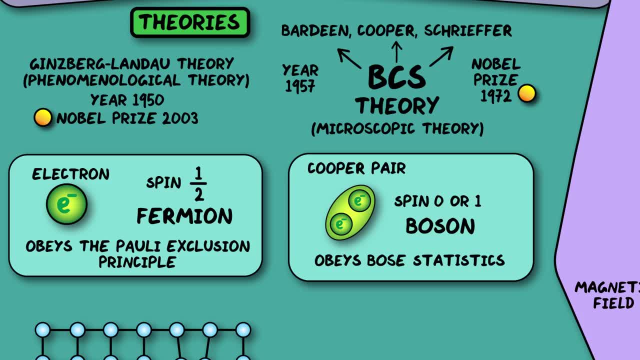 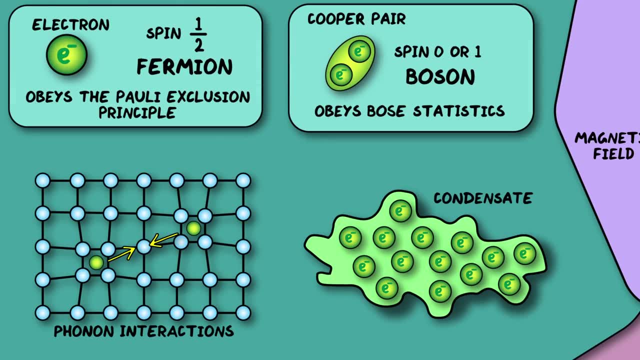 zero or spin one. bosons can exist in the same quantum state, and so all the cooper pairs form a superconductor, called a condensate, which has special properties, including not being able to easily absorb kicks of energy, and so they flow without resistance. this is known as an energy gap. 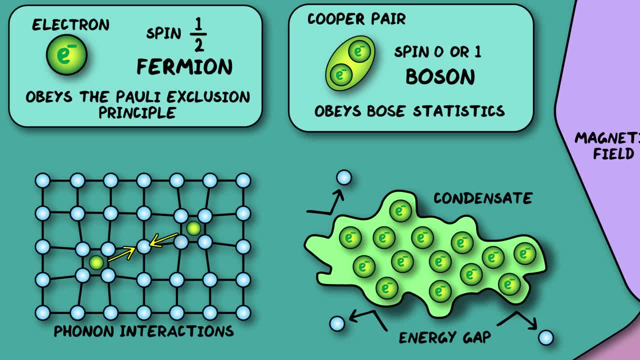 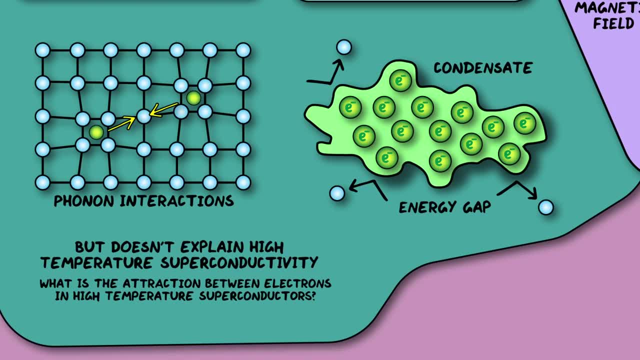 that's just a very quick explanation, because a full description would take a long time. but now you've got the basics. what is interesting is this theory doesn't explain high temperature superconductivity, because the attractive force from the phonons don't exist there, so they need 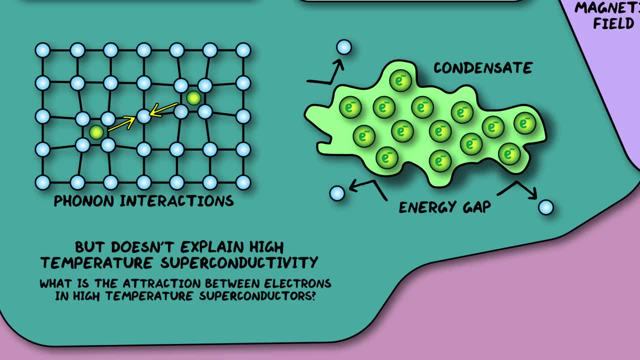 some other attractive force between electrons, and we don't know where that would come from in high temperature superconductors. for this reason, any superconductor that doesn't follow bcs theory is called an unconventional superconductor, and the ones that do are called conventional superconductors, despite a lot of 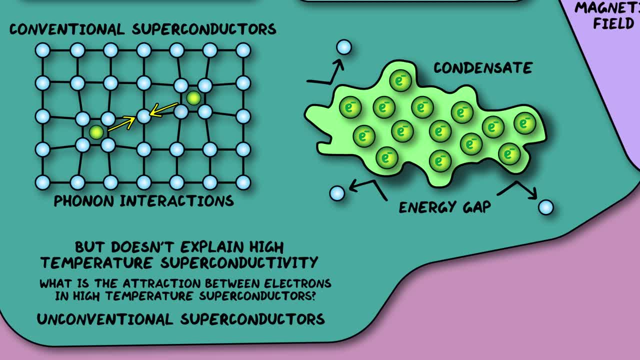 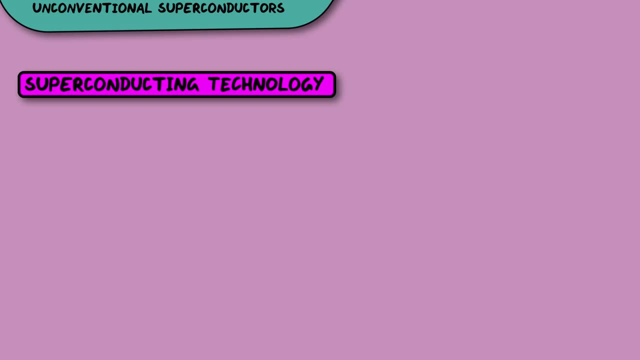 work going into this high temperature. superconductivity is still one of the biggest unsolved mysteries in theoretical condensed matter physics, and you'll probably win a nobel prize when you figure it out. there are a load of technologies which use superconductors to achieve this. the most widespread use of superconductors is to create: large magnetic fields, as you can circulate a lot of current in a loop without burning any energy. this is what the big tube is in mri machines. it's basically coils and coils of superconducting material that's cooled down with liquid helium. superconducting magnets are also extensively used. 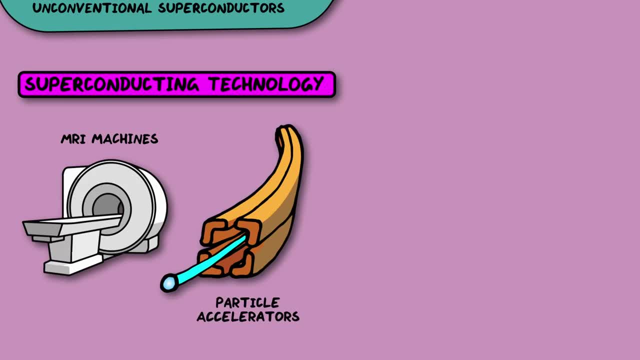 in particle accelerators to bend and focus the beams of particles. they've been used in some tokamak reactors to control plasma in the near right to the right area of the spectrum. that's actually the most powerful superconductor in the plus field of our human cells, which is the more 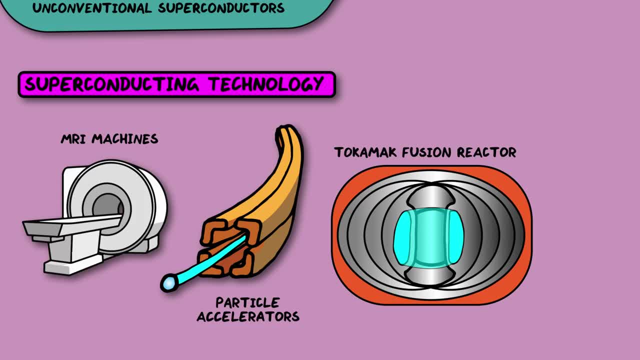 powerful, the more powerful, the more powerful the superconductor in the near right is. they are all fundamental. so, in general, all the matter that's going to increase is going to be better, if that's what they're lack in the, the nuclear fusion process and also in other areas where you want to control charged particles, like 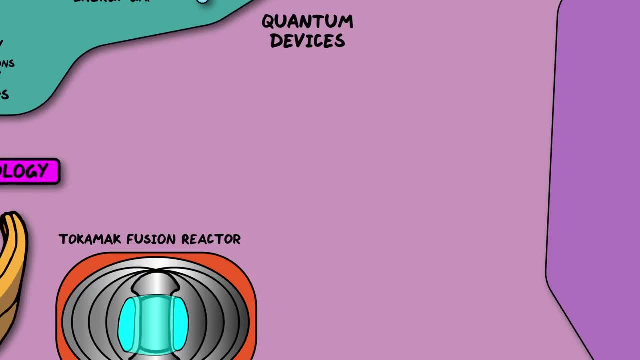 mass spectrometers. There are also many kinds of quantum devices which use superconductors. The most useful are Josephson junctions, which are small gaps between superconductors where the cooper pairs can still flow across the gap through quantum tunneling, and so you get a continuous flow of current even with no voltage applied. You can use this to set 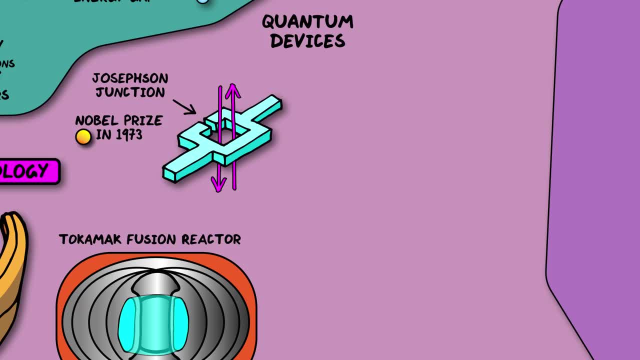 up superpositions of current and therefore superpositions of magnetic field, where the current and magnetic field are in the superposition state of flowing in both directions at the same time, These Josephson junctions can be combined in a specific formation called a superconducting. 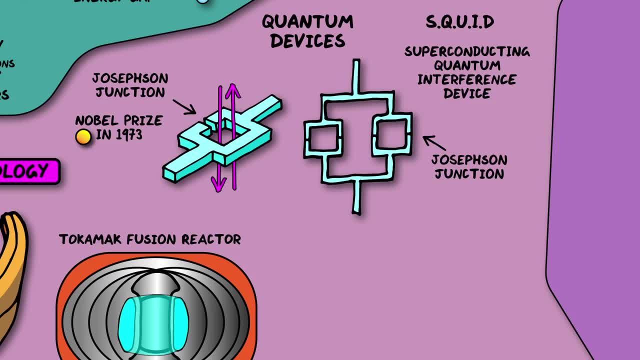 quantum interference device, or SQUID for short, which is a phenomenally sensitive magnetic field detector- the best humanity has discovered. These are the detectors that can see inside your body. in MRI and MRI They're also what set the voltage standard in fundamental physics. They're used as efficient. 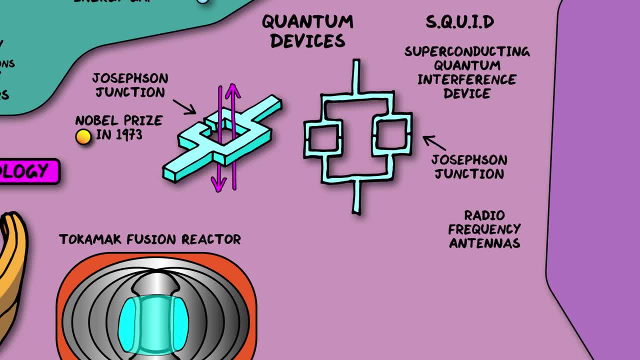 radio frequency antennas in research and in mobile phone masts, and you can use the superposition of states created by the Josephson junctions to make a tunable qubit, which are the building blocks of superconducting quantum computers. This stuff is my professional background back. 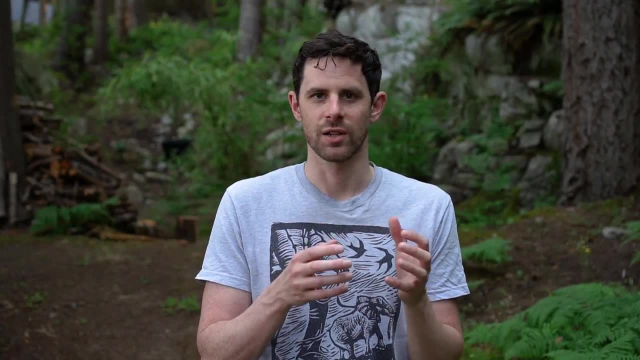 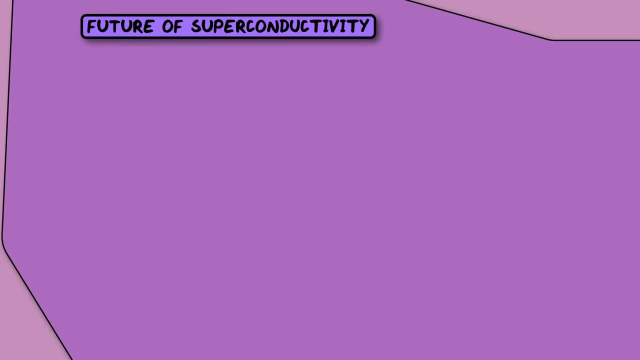 when I had a proper job, and I think quantum technology is absolutely fascinating, especially the possible future technologies. So what does the future hold for superconductors? For a long time people have talked about building transmission lines to transport electricity through superconductors to significantly reduce the amount of energy that's lost But to be cost effective. it. 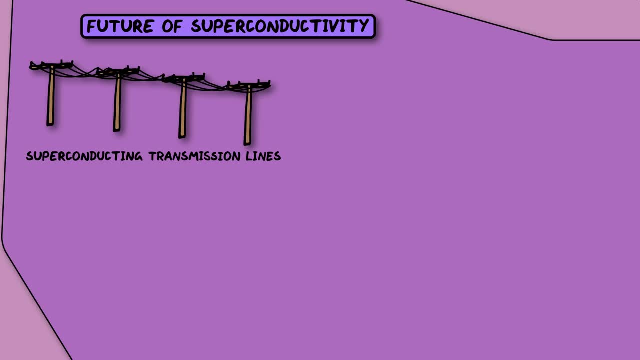 would need to be a superconductor that you don't need to cool down very much, which can carry high currents and is strong. We don't have this yet. so these are the challenges, but it would be cool to be able to ship electricity around the grid a lot faster than a superconductor would. 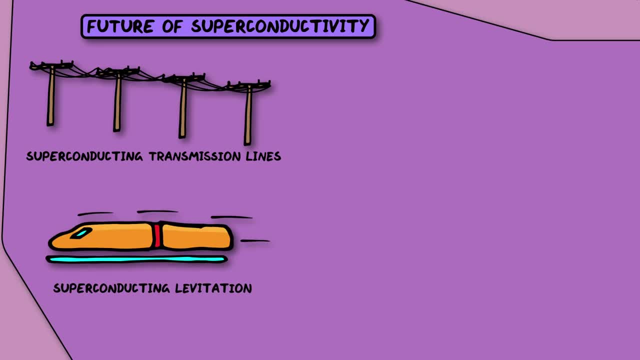 more efficiently. You can also use superconductors for levitating things like trains, but this potential has been around for a while, so I'm not sure there's a great need for it. but you know, it's a thing that exists. A promising area is to make very efficient superconducting motors or generators. 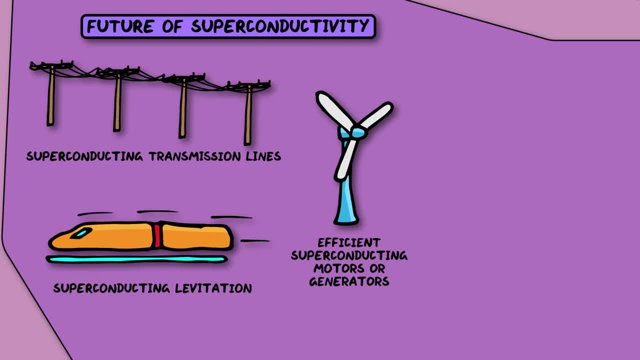 for things like wind turbines, which could potentially decrease the cost of the electricity they generate. So this would be really cool to make renewable energy even cheaper. On the quantum devices side, I think by far the most expensive way to build a superconductor would be to build a 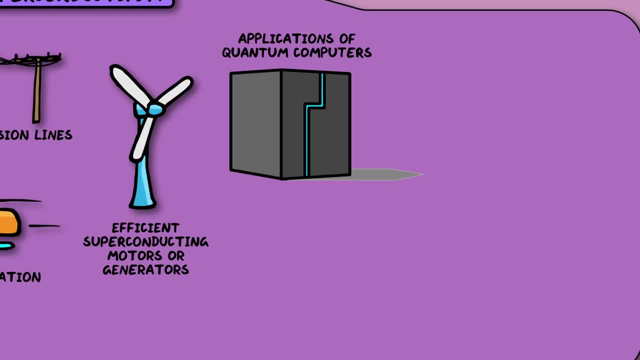 superconductor that would be more efficient than a superconductor that would be more efficient than a quantum computer. The most exciting applications are the range of quantum computers built with superconducting qubits. Now, superconductors aren't the only way to build quantum computers. 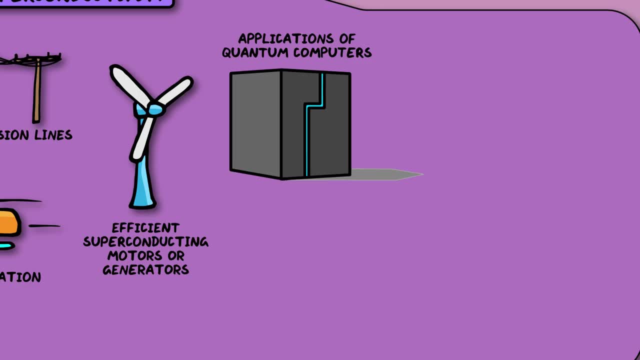 but Google, IBM, D-Wave and others have built very advanced superconducting quantum computers which could potentially be used to understand and find new superconducting materials by simulating the quantum mechanics of them, Something that currently can't be done with our most powerful supercomputers. So you could potentially use superconducting 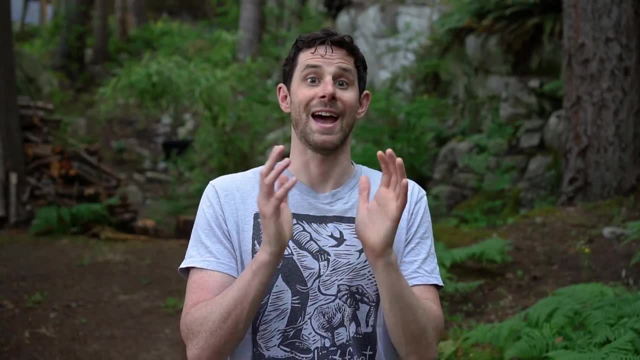 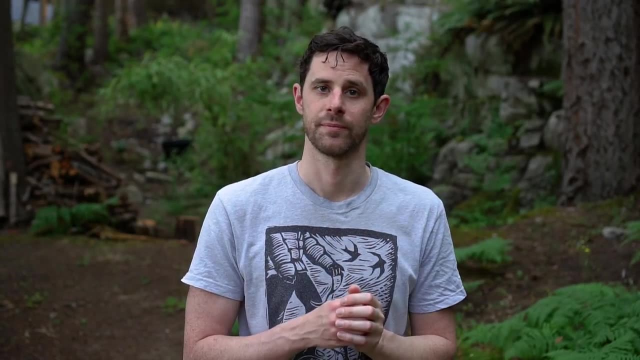 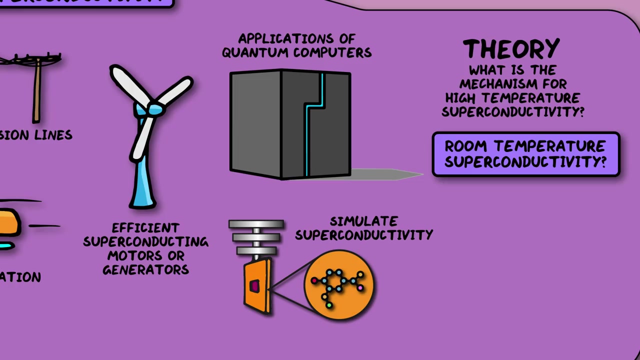 qubits to figure out how high temperature superconductivity actually works and then perhaps use that to find a room temperature superconductor. In fact, on the research side, figuring out the mechanism of high temperature superconductors and whether a room temperature and room pressure superconductor can exist, would be fantastic If we had a room temperature.